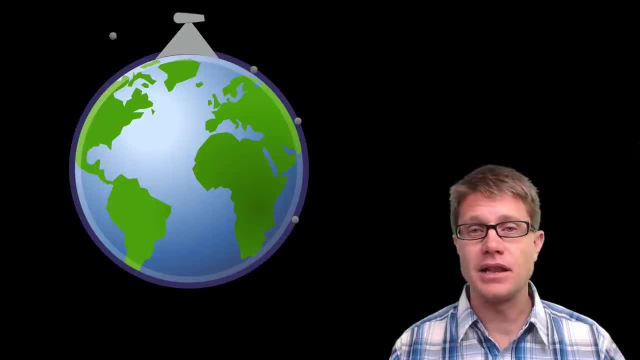 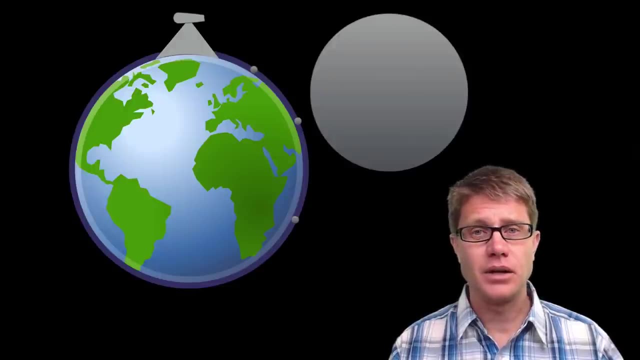 just keeps missing it, And so it is going to orbit around the earth. This is how satellites work, And Newton predicted this years ago. And so what would it feel like to be inside that cannonball? Well, you would feel weightless. It is not that there is no gravitational force. 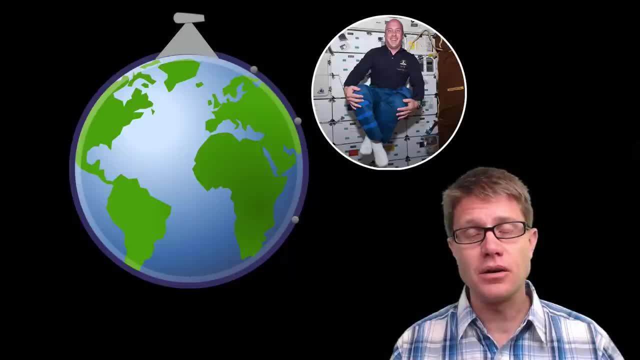 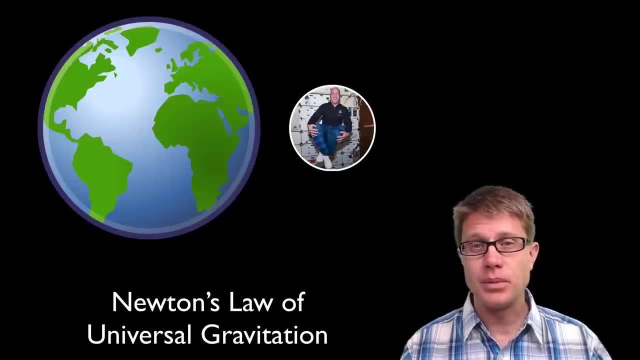 there, It is just as big as it was before. It is just that, as you fall towards the earth, you keep missing it. And so again, Newton's law of universal gravitation allows us to not only understand this, but to quantify it, To come up with 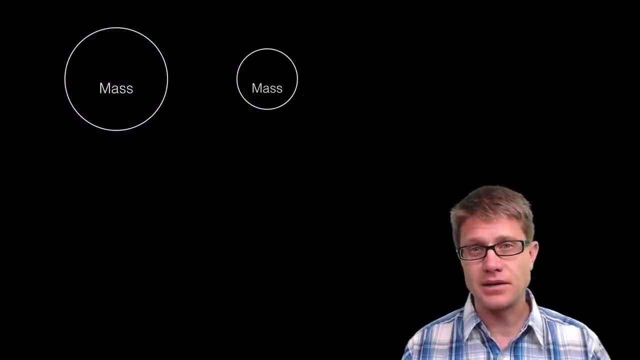 a value for that, And we are going to do that in this video. So if we have two masses, there is going to be a gravitational force between the two, And that is always going to be attractive. with anything in mass. Let's just assume that these are spherically symmetrical objects. 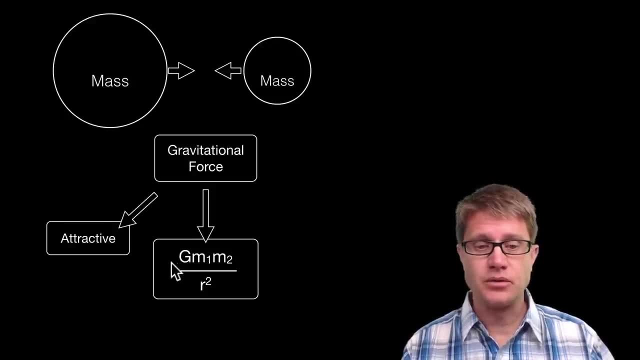 The equation is really, really simple. It is simply: the force is equal to big G- and we will get to that in a second times- the mass of the two objects divided by the square of the distance between the two. So you simply calculate the force by multiplying the masses. 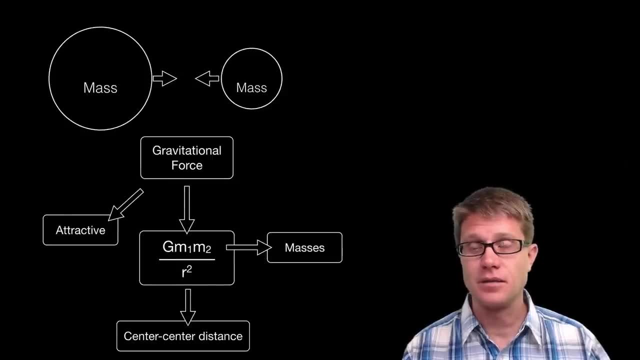 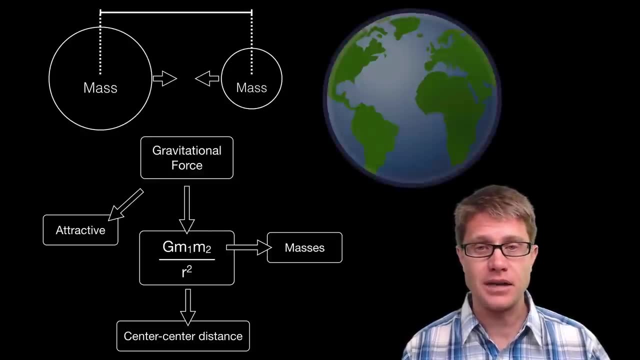 times this constant And then you divide it by the center center distance. But you are going to square that value. Center, center distance is always going to go to the center of those two objects, or the center of mass. Now on our planet, the earth is so big in relation. 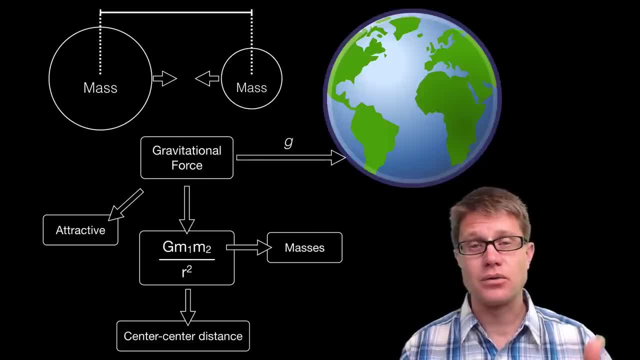 to us that this gravitational force or this gravitational acceleration- we will call it G- is essentially constant. Changes in our distance from the earth are so small that the mass is so big in relation to our mass that it really does not change much over time. 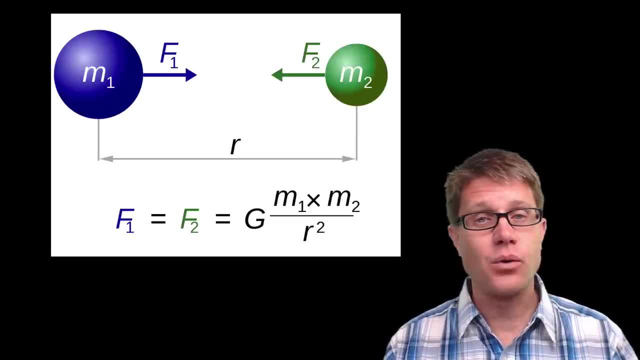 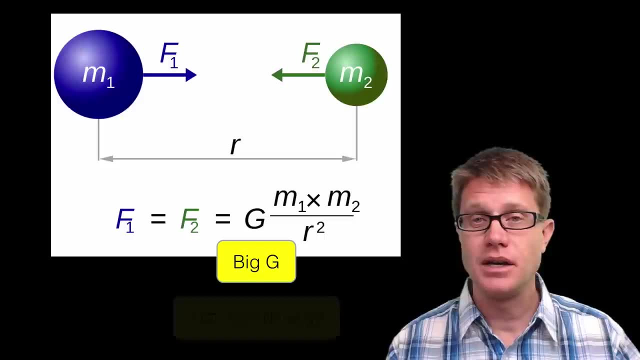 And so here is our equation: We have two objects, Then the force is going to be equal between the two, And it is explained using this equation right here, where G- we will refer to it as big G- is a constant, And it is worth memorizing. It is 6.67 times 10 to the negative 11th. 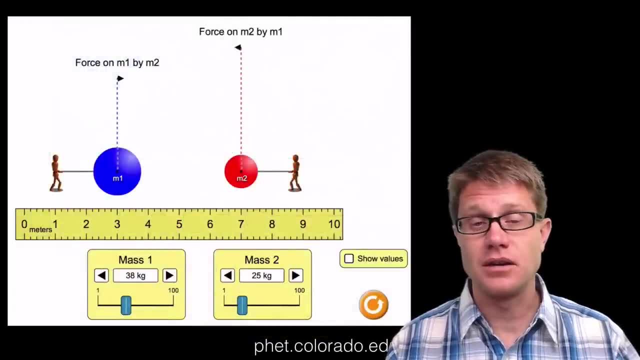 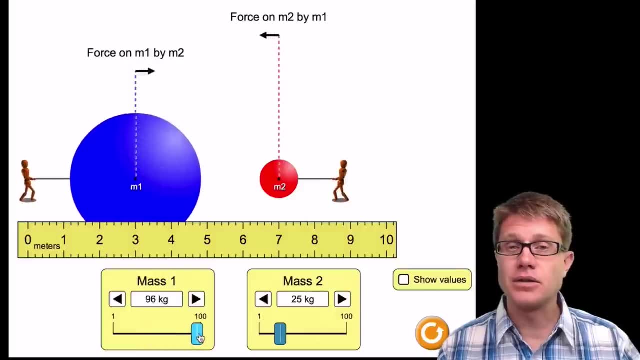 And so what else do we have in this equation? It is the mass of the two objects and then the center, center distance, And so there is a nice PHET simulation that gets at that. So if I have two objects like this and I increase the mass on one, you can see the force is. 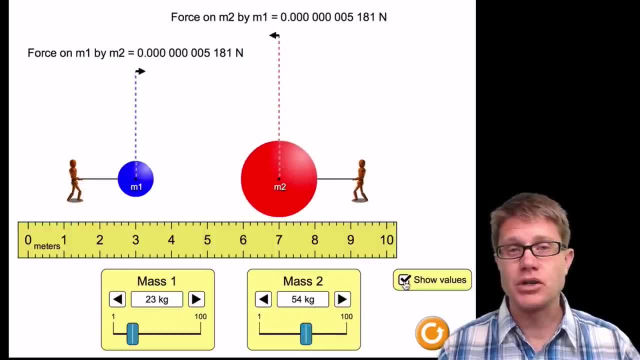 increasing on both of them And the force is always going to be equal. Now, if we show the values, you will see that those numbers are incredibly small. But what happens? as we move them close to each other, The force gets larger. As we move them apart, it gets. 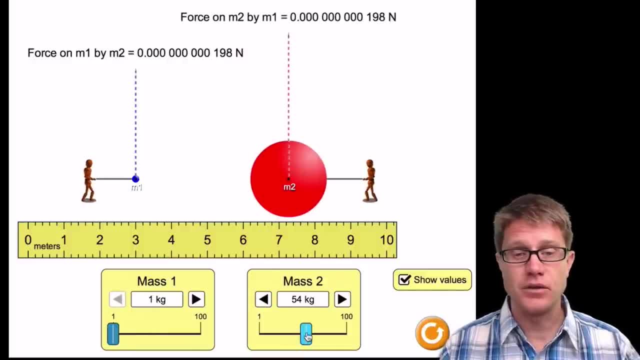 smaller And we can start to do some actual analysis here. If we make both of their masses one to make the numbers easy, and then we move them one meter apart, you start to see that gravitational constant come out. It is a really small value. It is a really small. 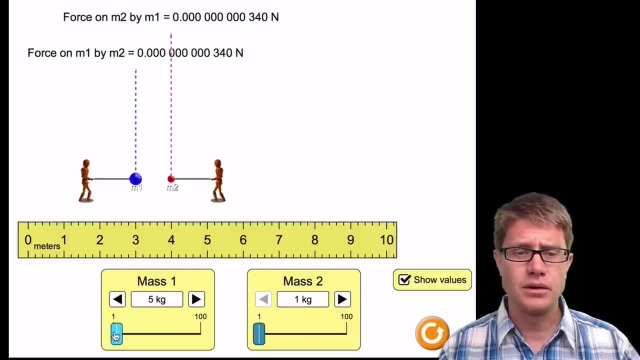 value. What happens now if we increase the mass tenfold? So if I increase this to 10 kilograms, you can see the force increases by 10.. What if I increase this mass by 10? We also see a tenfold increase, But it is not the same. if we are looking at the distance, 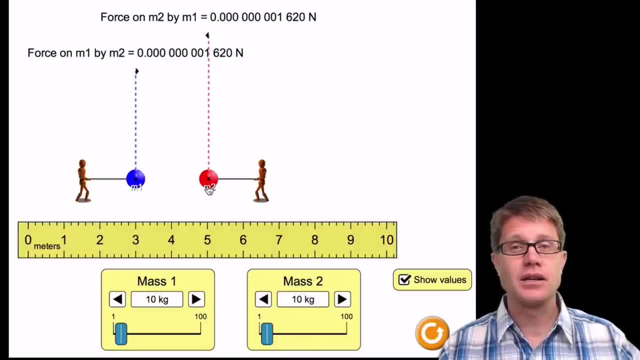 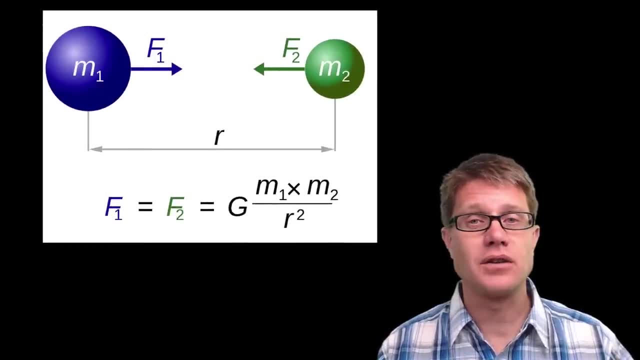 If I double that, we are not just cutting it in half, We are taking it by a fourth, And that is because we are squaring that distance between the two. And so, if this is our equation, let me show you how to solve a simple problem, And this is what you might see in a physics. 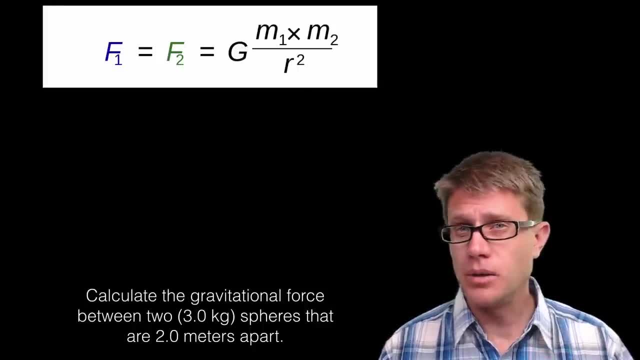 class: Calculate the gravity of the object. Calculate the gravity of the object. Calculate the gravitational force between two 3.0 kilogram masses that are 2.0 meters apart, And so this is going to be a really small value, hopefully when you get it. And so we know the gravitational. 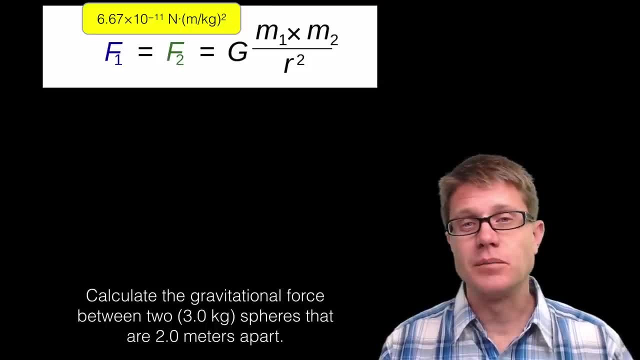 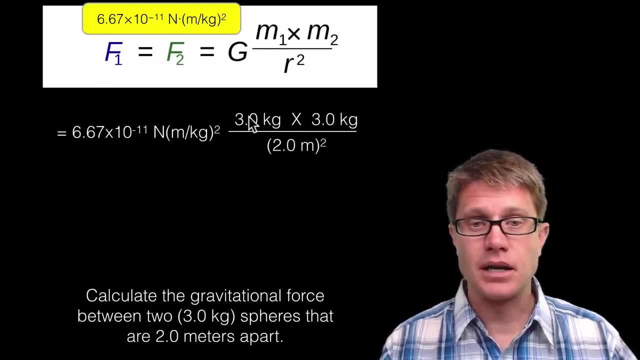 constant is 6.67 times 10 to the negative 11th. I am given the masses and the center center distance, And so it is really easy to solve that. I have got my constant g. Then I am going to multiply my two masses on the top And then divide that by my center center. 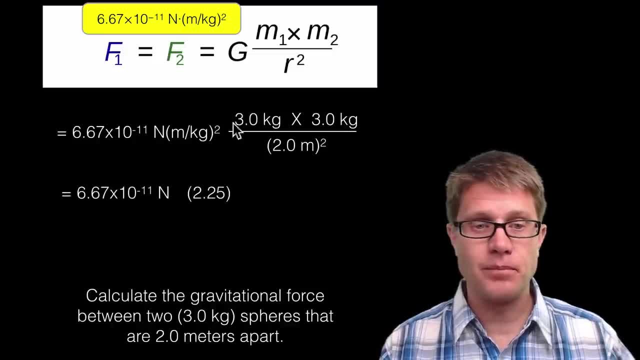 distance squared, And so, if I simplify that a little bit, my constant is here. What happened to these units? Well, you can see that I have got kilogram squared on the top and kilogram squared on the bottom here. So those cancel Meter squared on the bottom, Meter squared on the top And 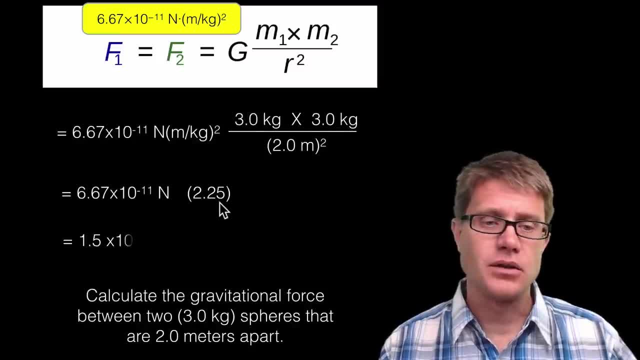 this is simply 9 divided by 4, which is 2.25.. And so what is going to be my force? 1.5 times 10 to the negative 10th Newton. So it is an incredibly small value. Let me give you a. 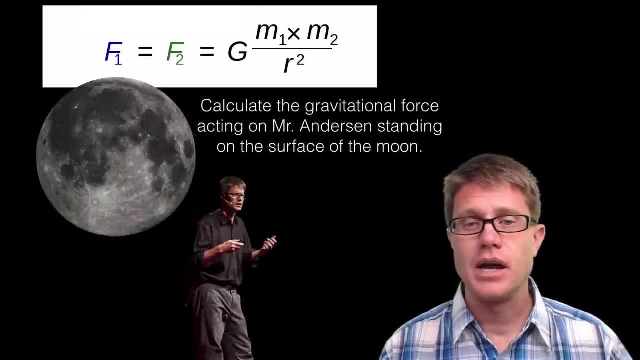 problem that I would like you to answer. So calculate the gravitational force acting on me Standing on the surface of the Earth, And then I am going to multiply that by the force of the force Standing on the surface of the moon. And so, if you are given a problem,